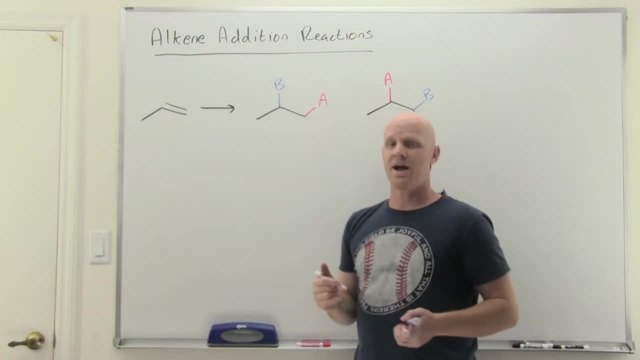 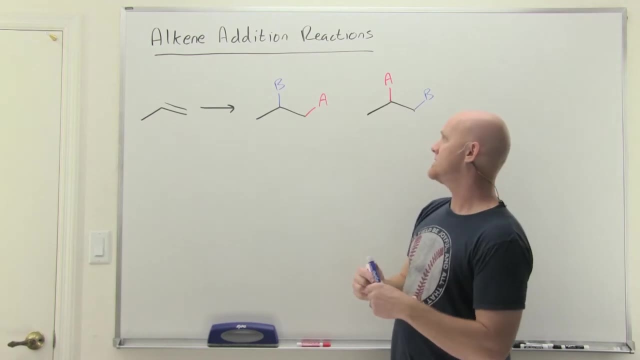 possibility of these two ways and we'll find out that. for you know, most of these reactions, they end up with two different groups and they prefer one of these over the other. So it turns out, in the first step of the mechanism of all our alkene reactions, the alkene is the nucleophile. 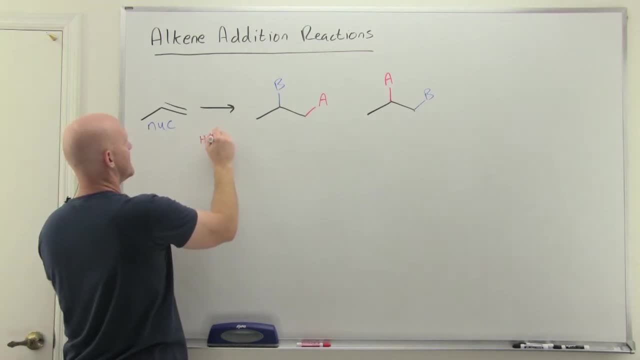 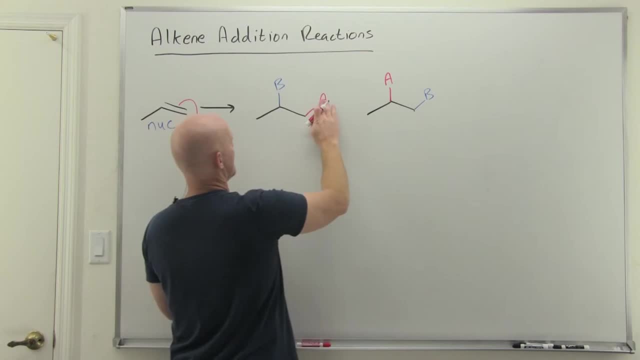 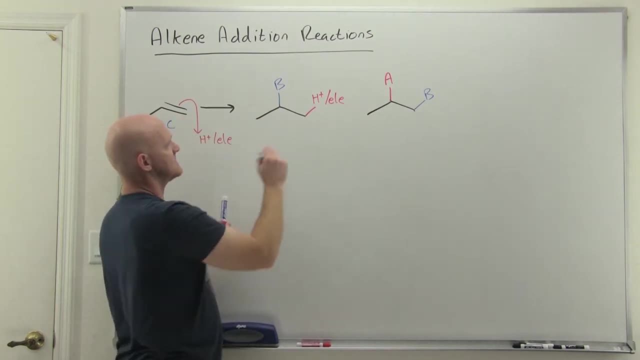 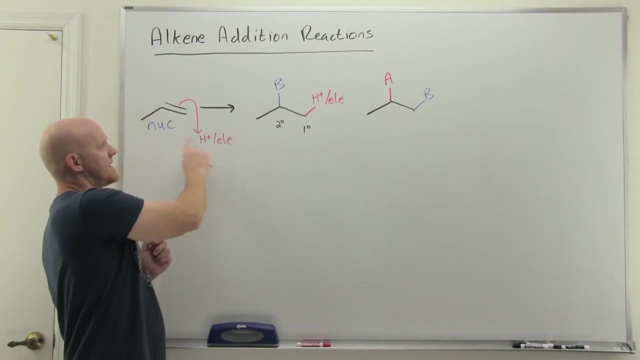 it does, so it turns out, majority of the time that's going to end up on the less substituted side of the alkene. So notice this is a primary carbon, this is a secondary carbon and the less substituted primary carbon is typically where the H plus or electrophile that gets attacked in the 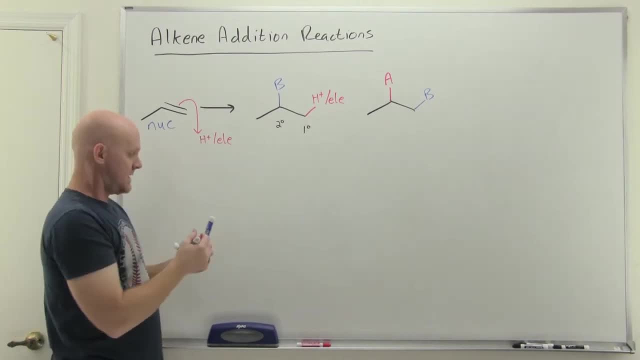 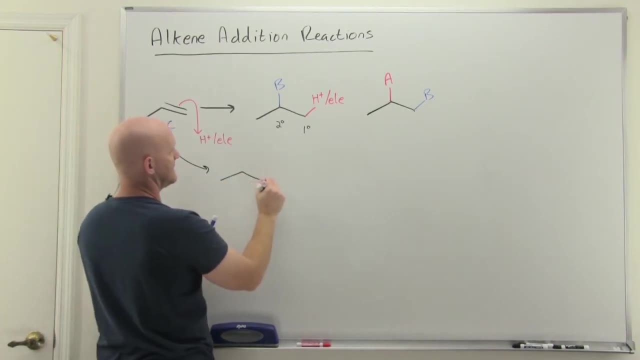 first step of the mechanism is going to end up. Now, it turns out, we can kind of see why this happens here. So it turns out the intermediate in a few of these reactions is a carbocation, And let's say we attached a hydrogen on that less substituted side. it leaves you with a 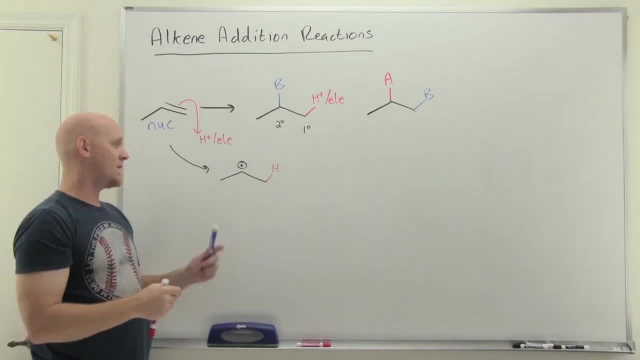 carbocation intermediate on the more substituted side. And so, had we done this the other way around- put the H on the secondary carbon- we would have ended up with a primary carbocation. But doing it the way we did, we ended up with a more stable secondary carbocation, And that's. 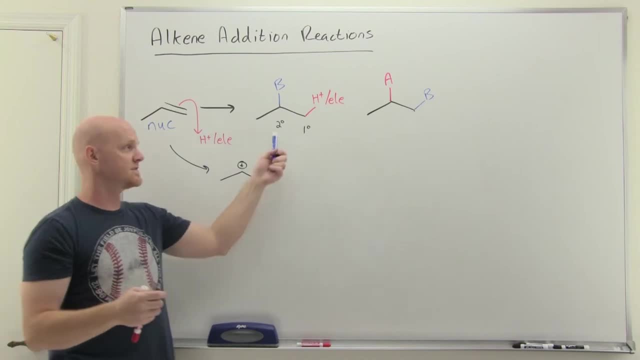 going to explain why we preferentially get one over the other of these two different regioisomers. Cool, It turns out in the next step a nucleophile is now going to come, attack the carbocation and attach there, And so B- here it turns out, is going to be some variety of nucleophiles. 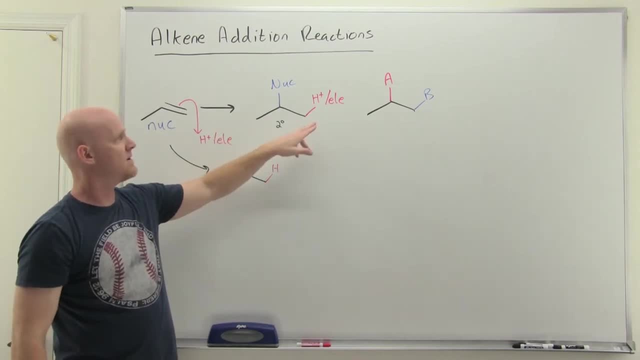 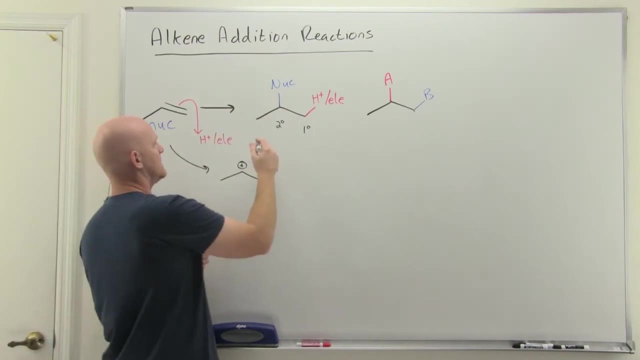 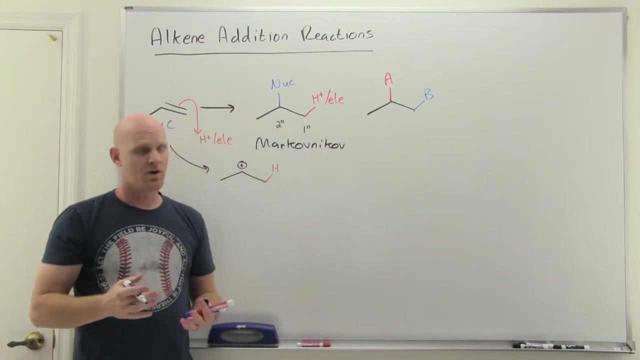 And we'll leave that generic here for a little bit. So and it turns out, as long as you add the hydrogen or electrophile on the less substituted side and the nucleophile on the more substituted side, you'll have accomplished what we call Markovnikov addition, So Markovnikov's. 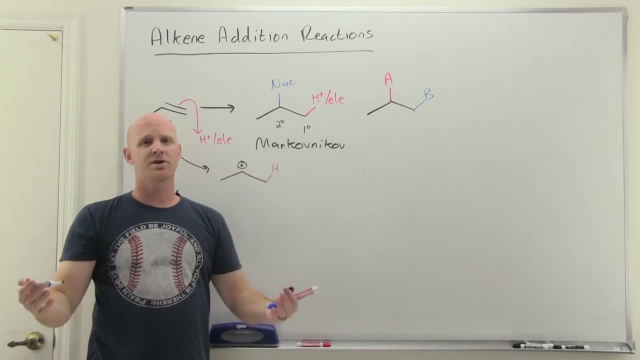 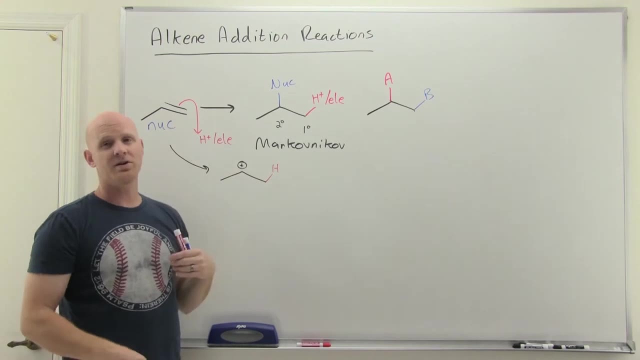 reaction, and this was the most common result, and we call it Markovnikov addition. Now you'll have to memorize who the either H plus or electrophile is for every single one of our sets of reagents, and therefore who the nucleophile is, And then you'll also have to recall, if it goes, 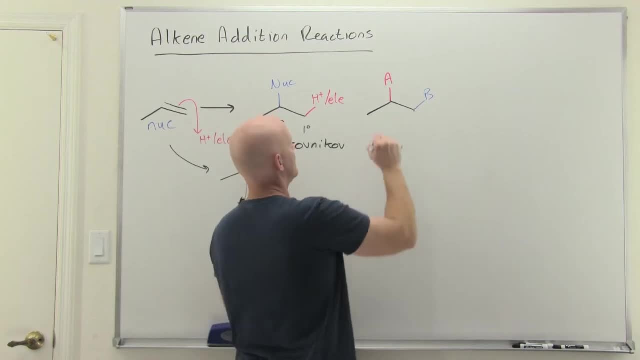 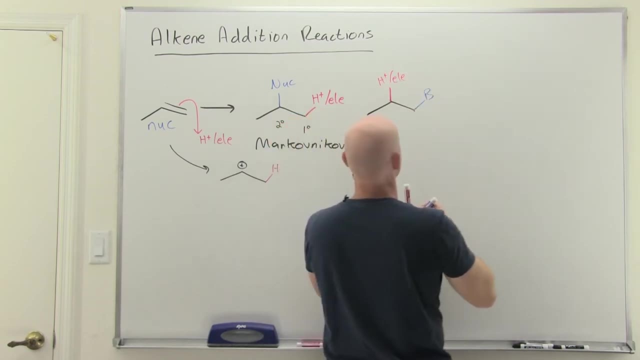 Markovnikov, or if it ends up doing the opposite. So in this case, A here again is H plus or the electrophile, and B over here the nucleophile, And this is way less common. In fact we're only. 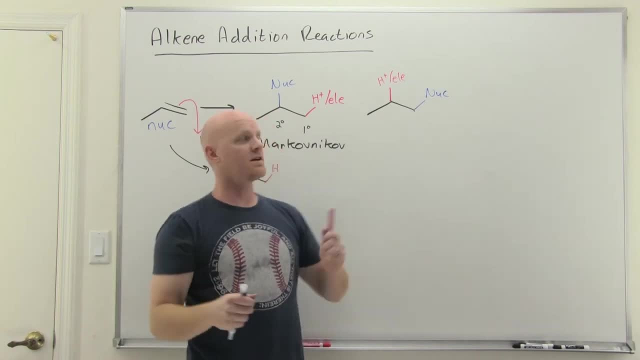 out of our like 15 reactions that will end up going opposite of Mr Markovnikov's rule here. So, and when it goes opposite Markovnikov's rule, we just call it anti-Markovnikov. We don't get. 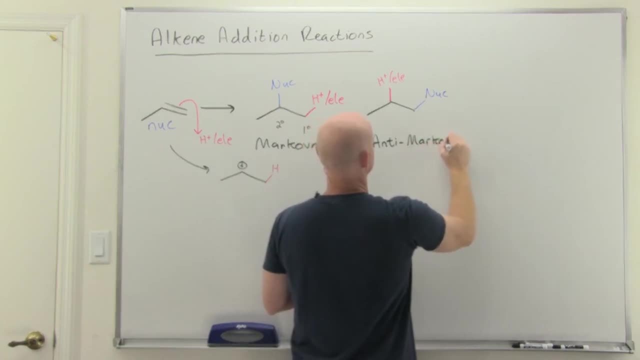 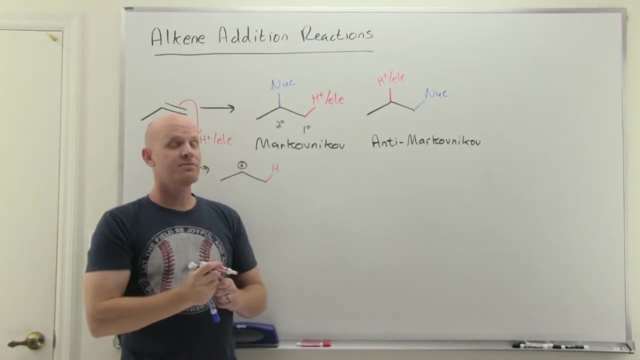 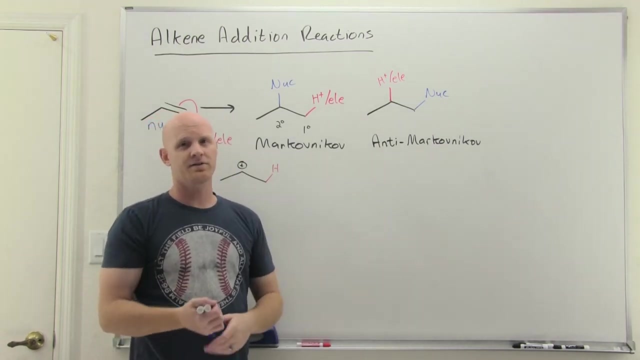 too creative on the name Cool. And so when a reaction goes either Markovnikov or anti-Markovnikov, we refer to that as the regioselectivity, because it's going to tell you preferentially which regioisomer is your major product And the vast majority of the reactions again are going to go. 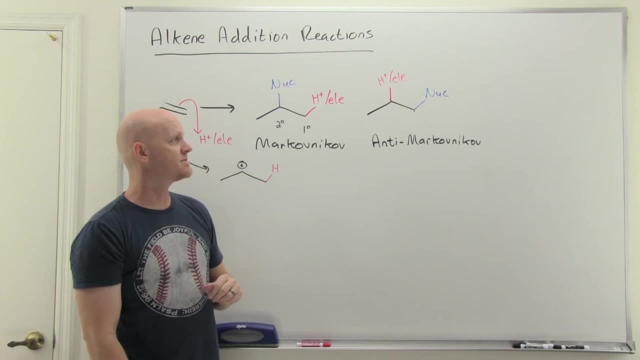 Markovnikov, but two of them- we'll study- will go anti-Markovnikov. Now we've got one more thing to talk about in this regard, and that's stereoselectivity, And that is: is there any relationship in the stereochemistry of the two groups that add? So, and before we get there, 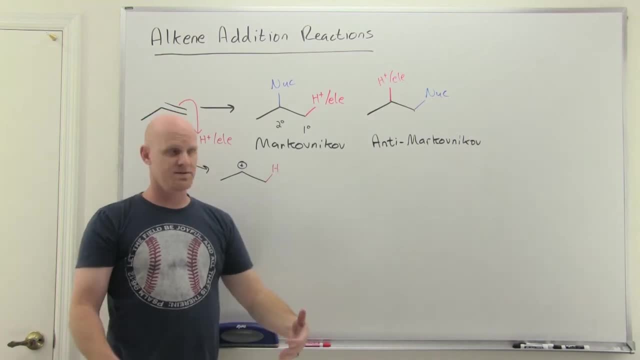 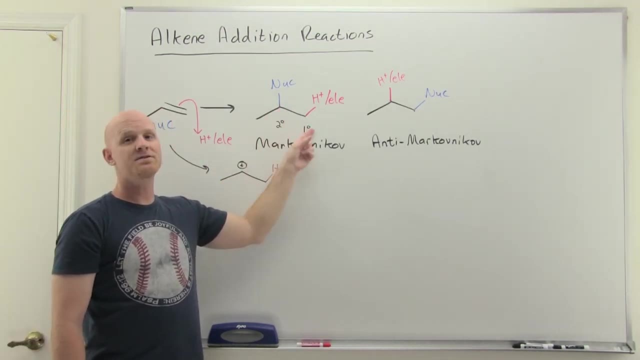 though we actually have to take this one other place to see why that's even important. So if we look at a reactant in an alkene, we've got two sp2 hybridized carbons that are about to turn into sp3 hybridized carbons, And that's important because those sp2 carbons they're never going to be chiral. 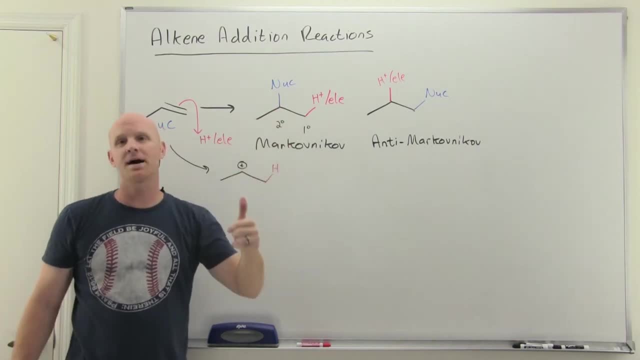 centers. So we've got two sp2 hybridized carbons that are about to turn into sp3 hybridized carbons. But in turning into sp3 hybridized carbons they might turn into chiral centers As a chance, being sp3 and tetrahedral. as long as they got four different groups, they're going to be chiral. 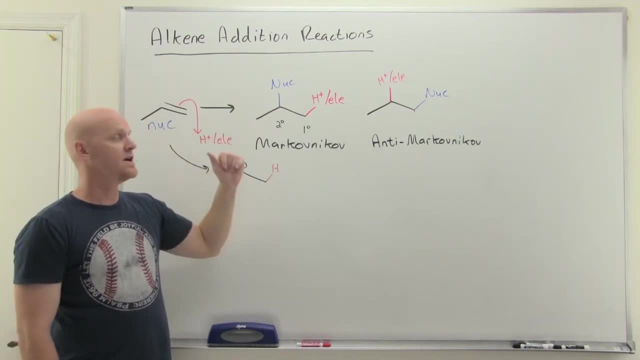 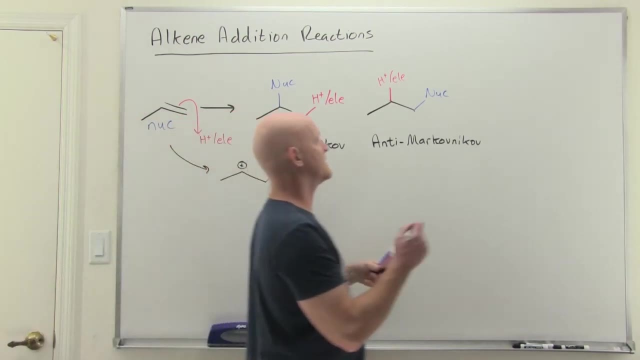 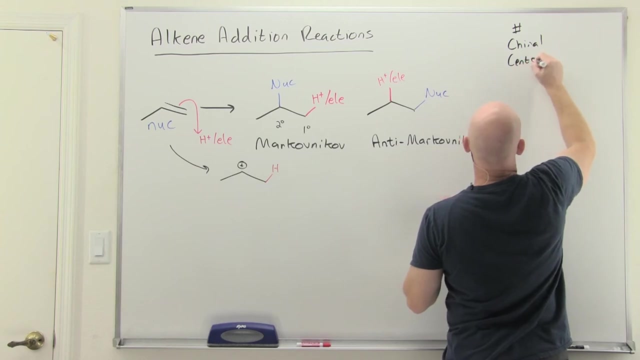 centers And so in a typical alkene reaction so you have a chance of forming up to two new chiral centers is typically the way it works. Now, if neither one of these turns into a chiral center, we can kind of classify this here. So let's say: number of chiral centers If you don't form, 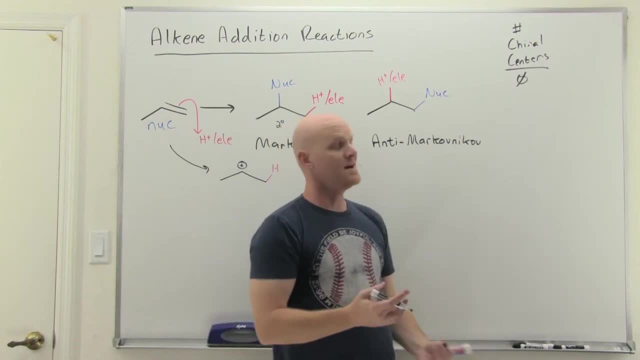 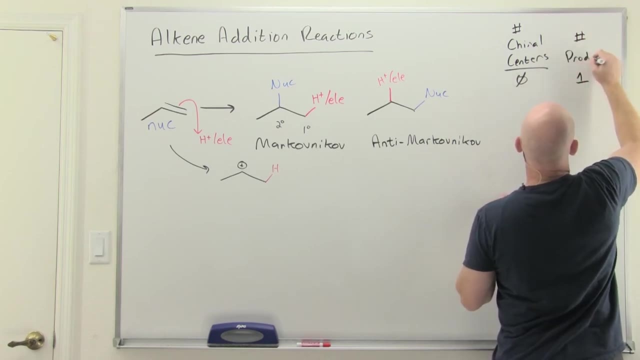 any. if those out of the two options you had, neither one turns into a chiral center, then you're just going to form a single achiral product, And so I'll label this as the number of products, And you just get the one achiral product, and life is good, Life is easy Now. 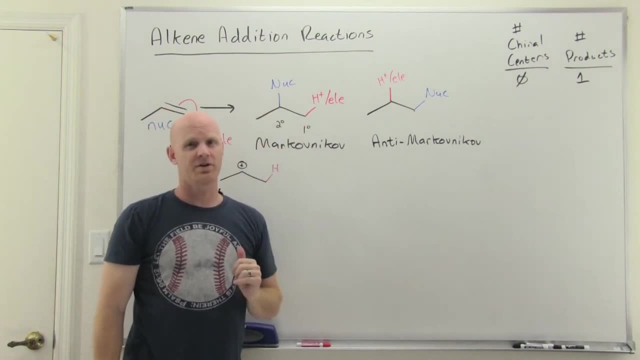 on the other hand, let's say, one of these two becomes a chiral center, So one out of two. Well, again, if you have one chiral center, it can exist as R or S And for every single alkene reaction. it doesn't matter any of the 15 that we studied, it doesn't matter any of the 15 that we 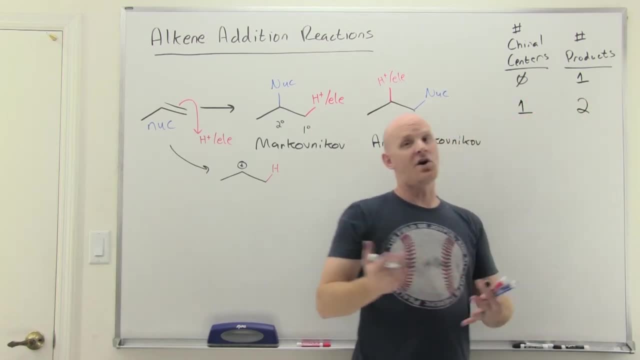 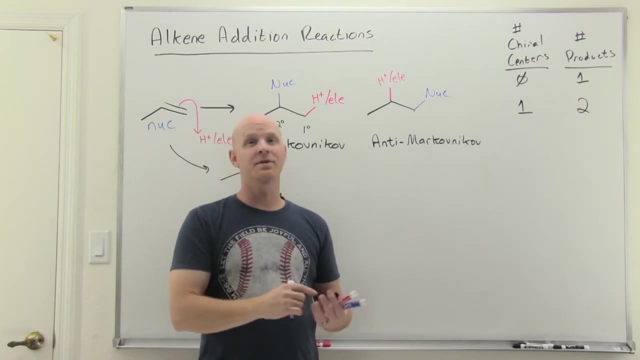 hear, If you get one chiral center, you're going to get two products- R and S- And if that's the only chiral center, well then those would be enantiomers, But if there are other chiral centers, then these might be diastereomers instead. But the key is you still get two products. 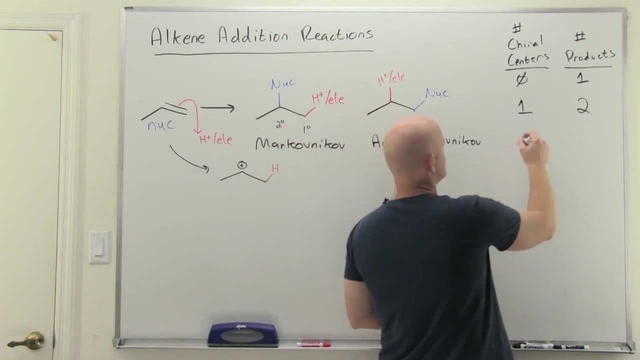 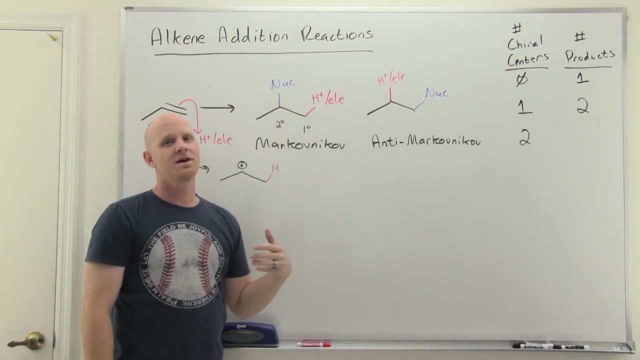 two different stereoisomers. What it gets tricky, though, is if you form two new chiral centers, if, where you add the electrophile and the nucleophile, if both of those turn into chiral centers, we have a problem. So, and the problem is that now you have a chance of getting up to 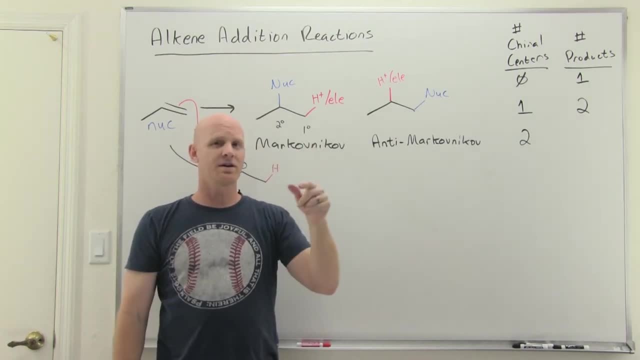 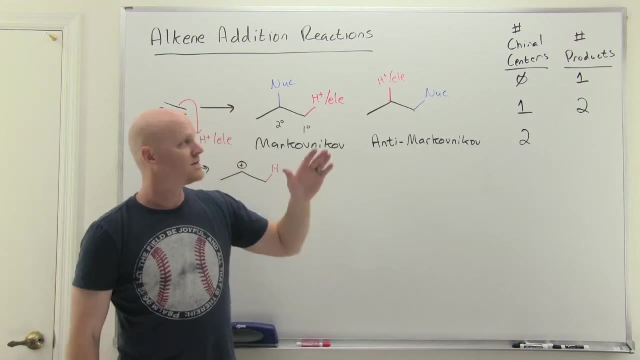 as many as four stereoisomers. So with two chiral centers you're going to get two products, chiral centers, two to the N, where two to the two. power is four different stereoisomers. It could be RR, SS, RS or SR. So with four possibilities, it really depends on the 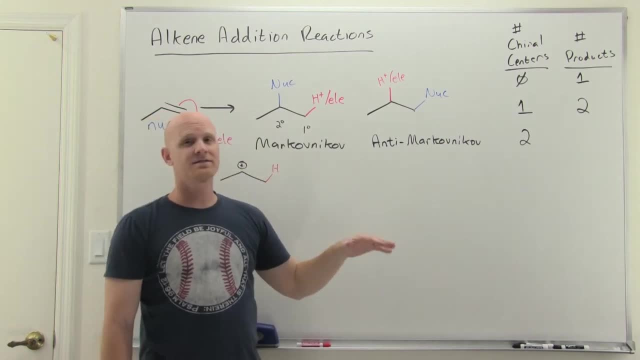 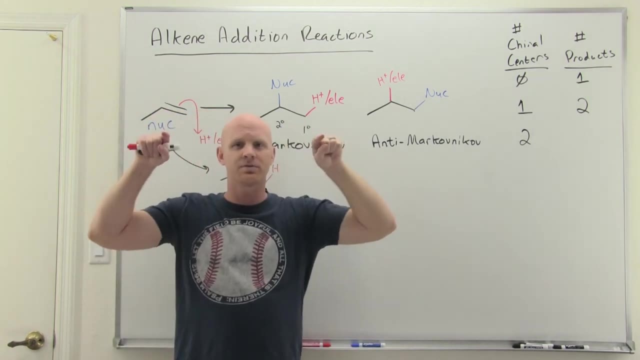 reaction now, And so it turns out when we talk about stereoselectivity, so there is in some reactions a relationship between the nucleophile and the electrophile, where they have to add to the same side both from the back or both from the front, In which case then you get two options. 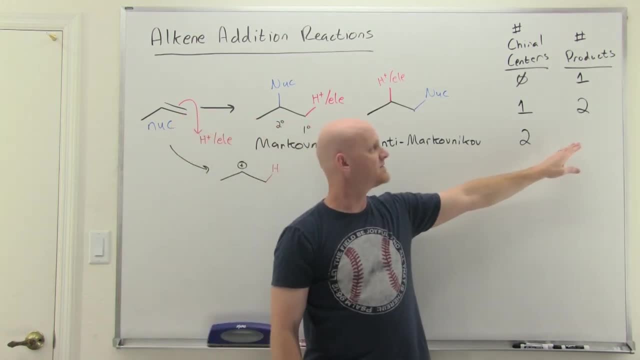 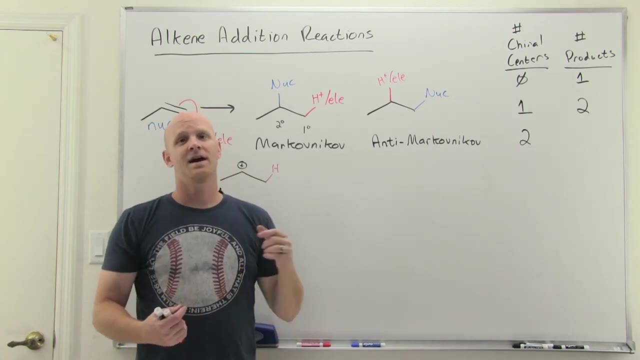 both from the back or both from the front, And out of the four possible stereoisomers that could exist when you have two chiral centers, you only get two of them. There are other reactions, though, that actually involve backside attack and end up with the nucleophile and electrophile adding from. 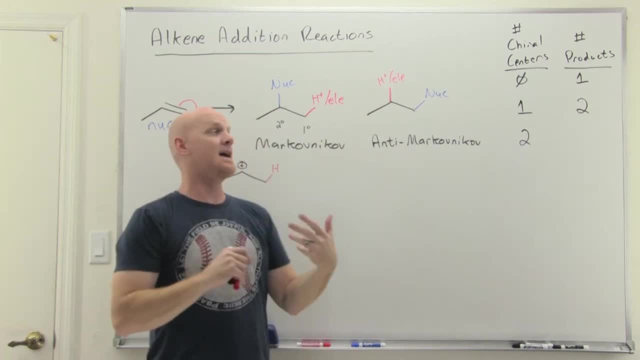 opposite sides, one from the front, one from the back, in one of two possibilities, And in that case we call that anti-addition. You only get two possible products. So if they added the same face front, both front or both back, we call that syn addition and you get two possible products. 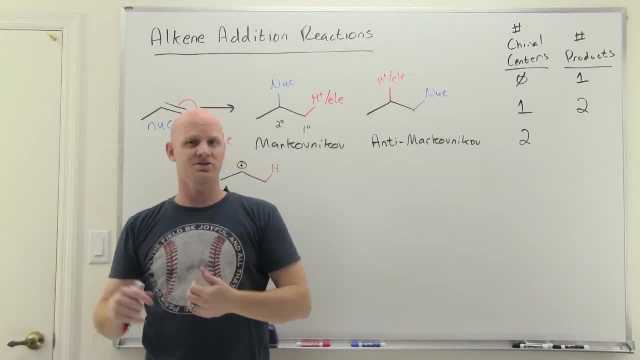 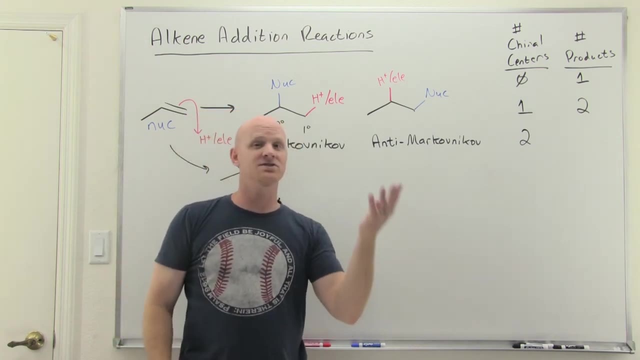 And if they add the opposite faces, you get two possible products. We call that anti-addition. And then you have the option where there's just no stereoselectivity whatsoever And you get both the two syn and the two anti-addition products. You get all four possible stereoisomers. 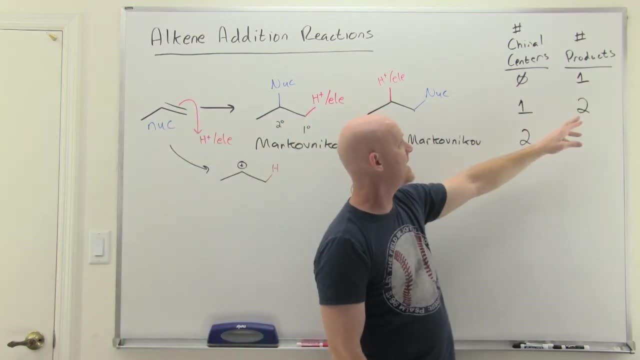 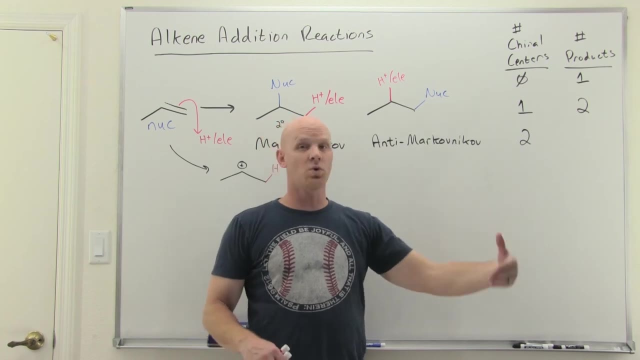 Now if you look at the little table on your handout, that's like this on your handout: it doesn't actually say number of chiral centers. It says number of chiral centers formed. So I don't- it's not the number of chiral centers in the whole molecule, just how many you formed when your sp2.